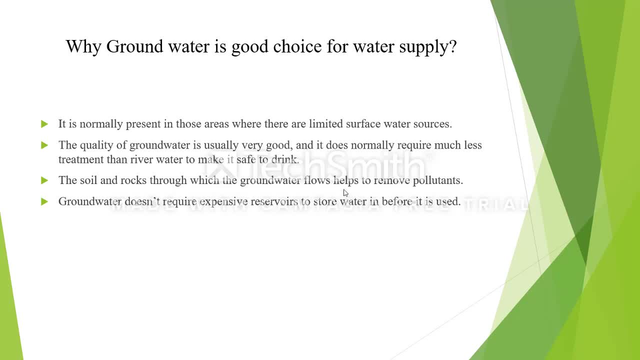 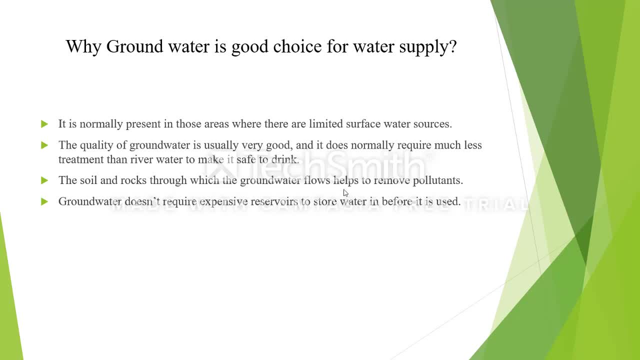 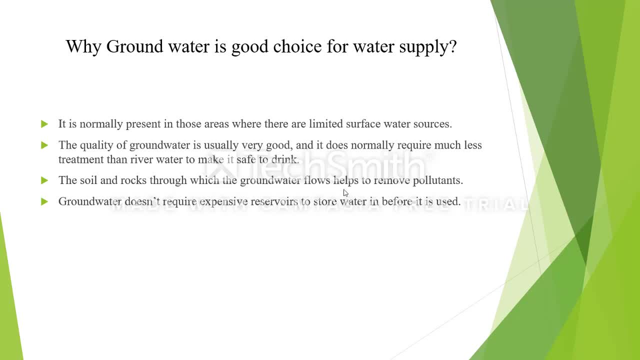 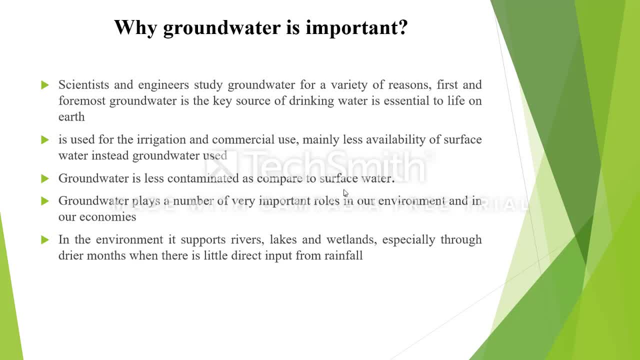 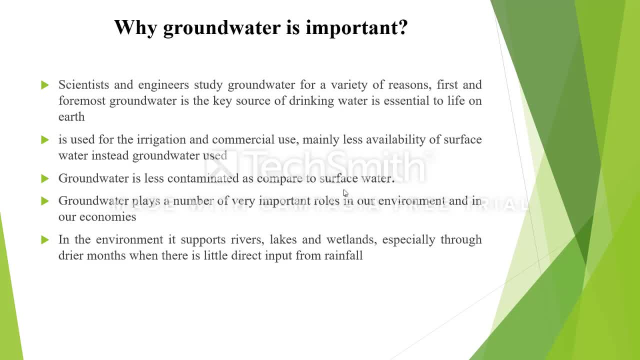 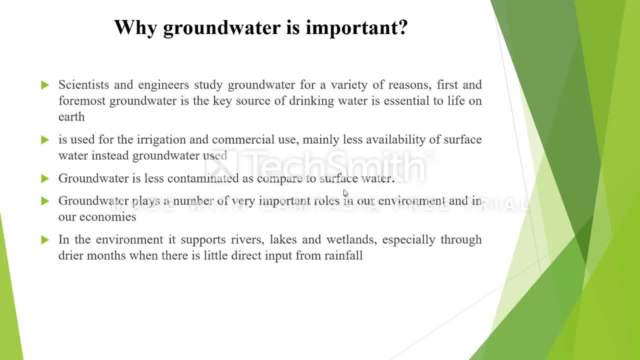 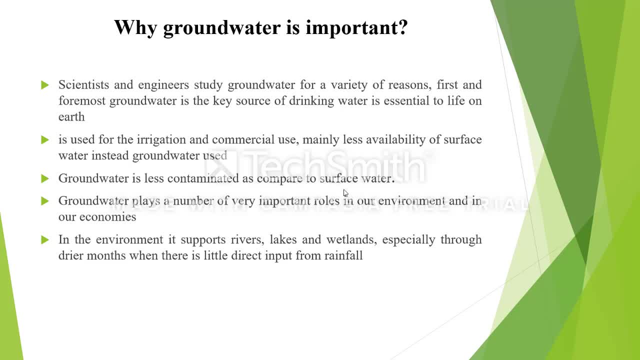 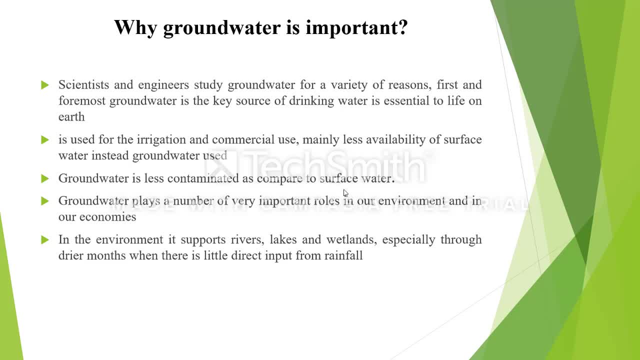 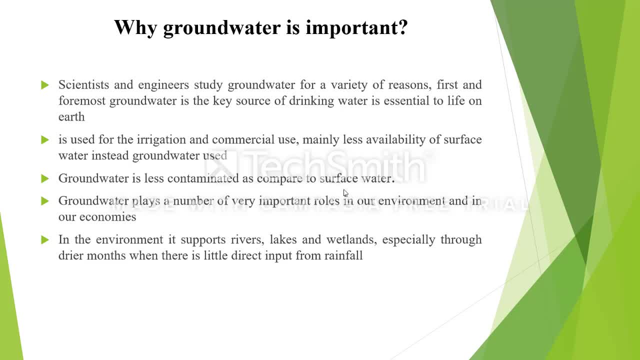 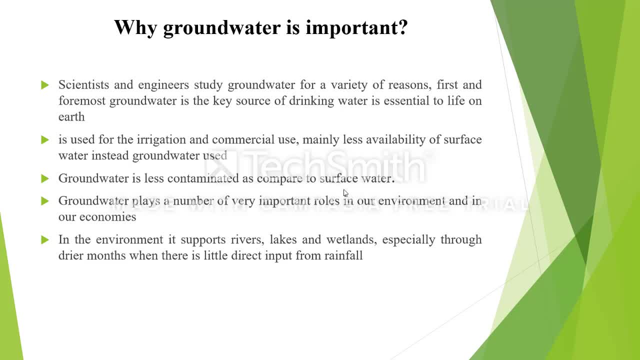 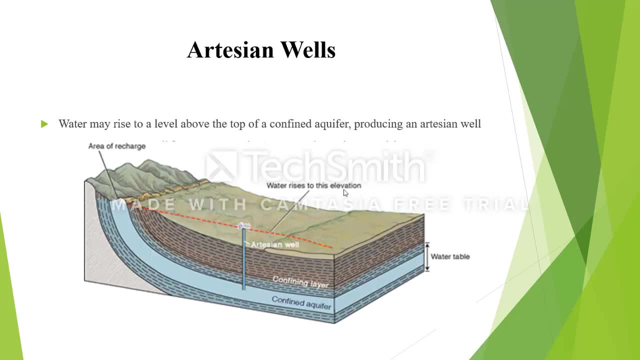 In the environment. it supports rivers, lakes and wetlands, especially throughout the drier months when there is little direct input from rainfall. Here is an artesian well. What is an artesian well? An artesian well? water may rise to the level above the top of the confined aquifer, producing 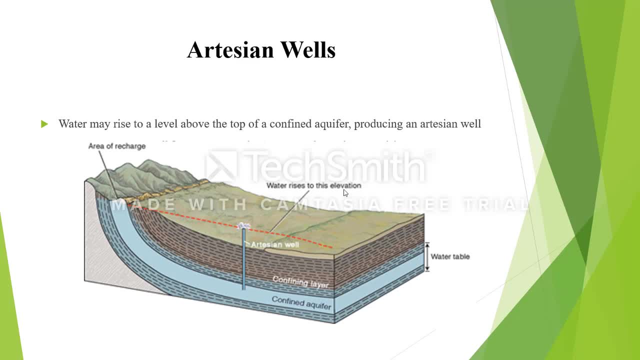 an artesian well. There are two types of aquifers. One is there are two or three types of aquifers, like the confined aquifer, an unconfined aquifer and an acuclude like these. So in this figure it shows area of recharge at the top and water rises to their levels. 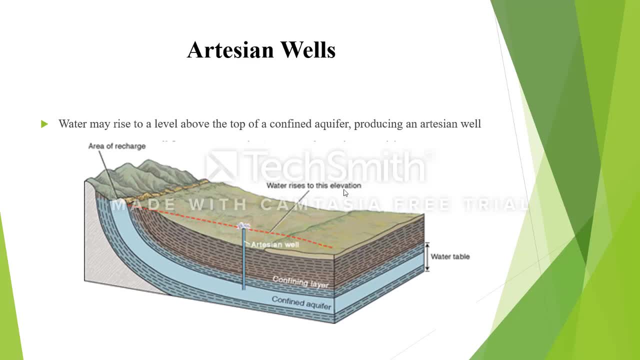 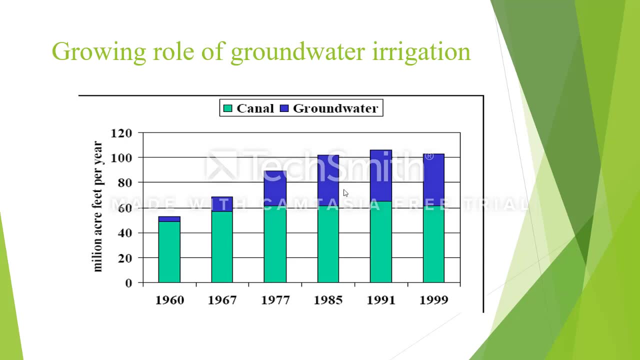 So when the water rises to levels and the water shrivels, that is called a artesian well Growing. role of groundwater irrigation in this graph mention the groundwater, how to development the groundwater extraction in yearly, in different years. So million per acre feet per year. we just mentioned the unit of the groundwater amount. 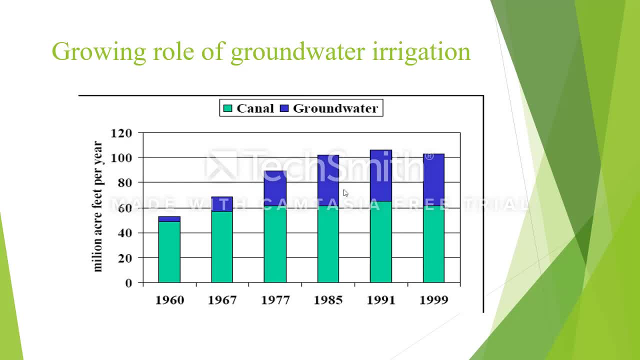 volume, So in 1960, here is green type color show that it's canal water. Blue color show the groundwater. So in yearly the groundwater extraction is more increased. In the period of 99, in this period the droughts occurred in this period, 99 to 2002, so people. 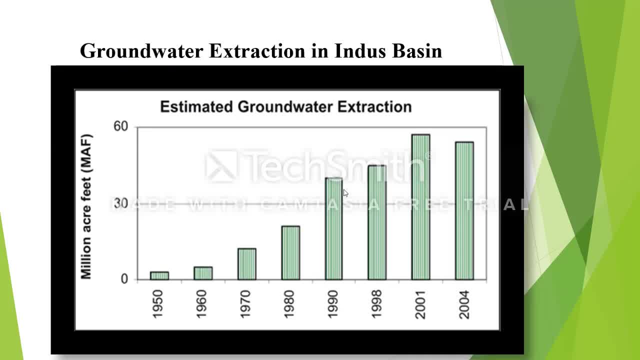 extract more groundwater in this period. So estimation, estimated groundwater extraction here is mentioned from 1952 to 2004.. So million acres acre feet, mf the unit, So groundwater is extracted in yearly more. It is increasing groundwater extraction because groundwater is used for a different purpose. 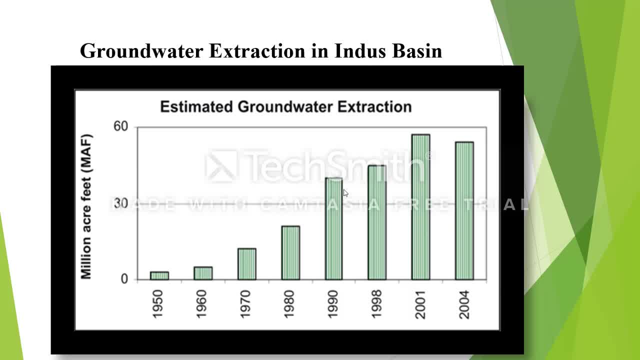 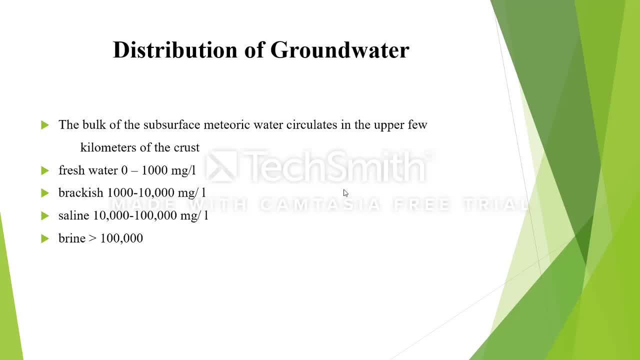 like that: irrigation and water drinking purpose like that in remote areas. So here, distribution of groundwater. the bulk of subsurface meteorite water circulates in the upper few kilometer of the crest. So what do you mean by meteorite water? 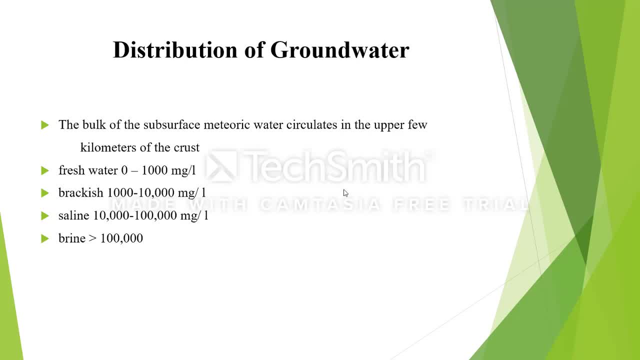 Meteorite water is the source which can water obtained from the precipitation silofa and other, So that is called meteorite water. So we normally just take them for irrigation purpose. Fresh water: 0 to 1,000 milligram per liter is studious. 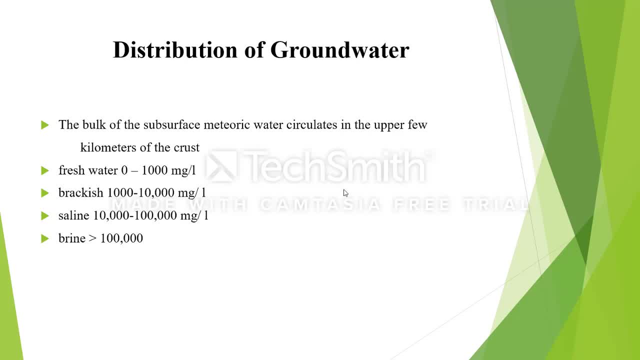 Brackish water: 1,000 to 10,000 milligram per liter. Saline water: 10,000 to 1,000,000 milligram per liter. In more than 1,000,000, the water is called the brine. Brine is impossible.